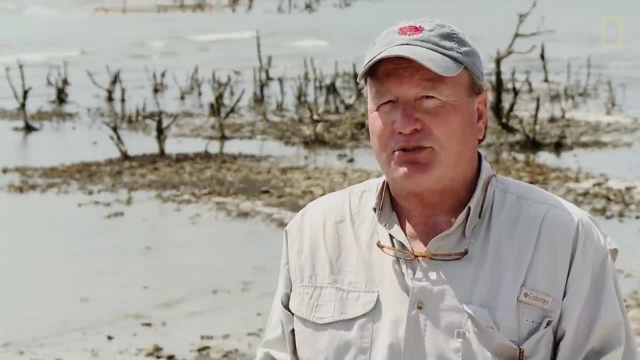 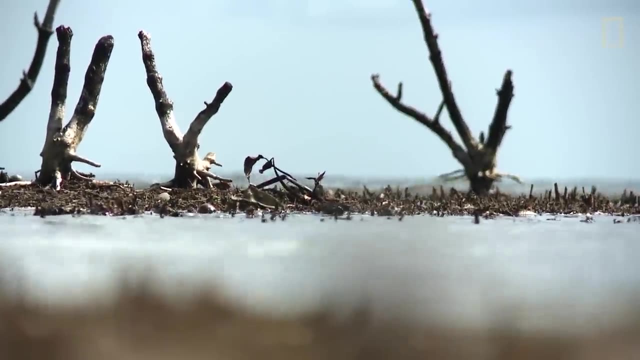 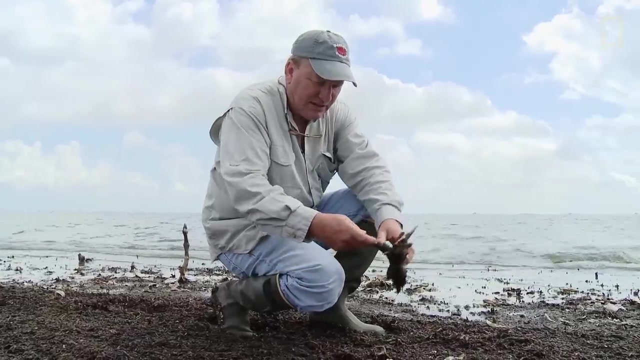 populations. We even had some rare and endangered birds that were actually nesting out here, and today nothing, They're all gone. There is an effort to restore this island and to bring sediment back and the mangroves back. so if we don't start doing restoration now in environments that were oiled, 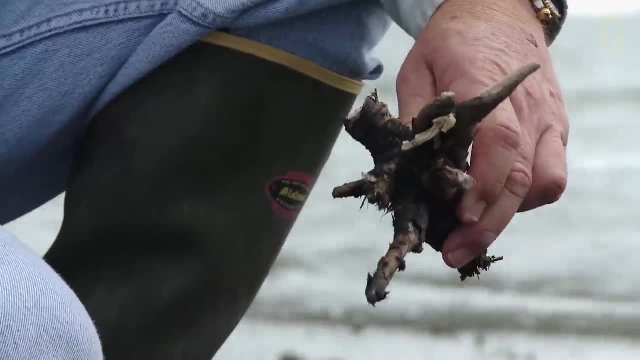 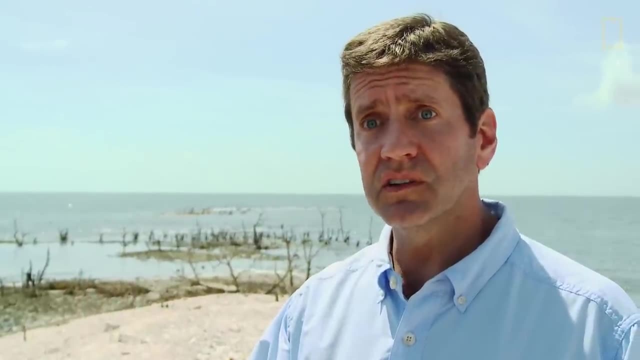 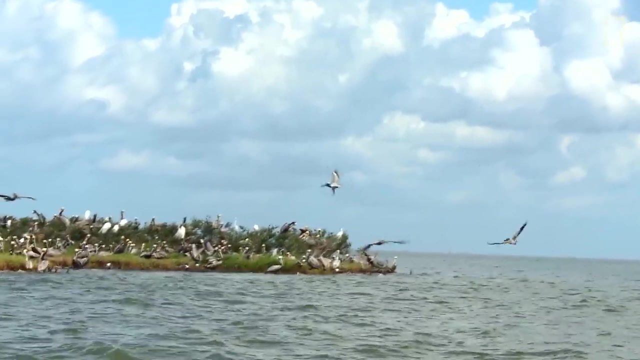 the harder that's going to be. It's going to take more resources, more money to build back what was there before the oil spill, Having this loss from sea level rise from natural erosion and to be exacerbated by the BP oil spill. to me, it really is, in a way, the canary in the coal mine, for the habitats that are going to be threatened in the next couple decades. 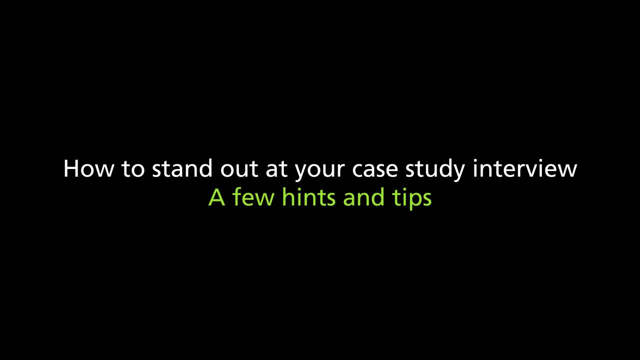 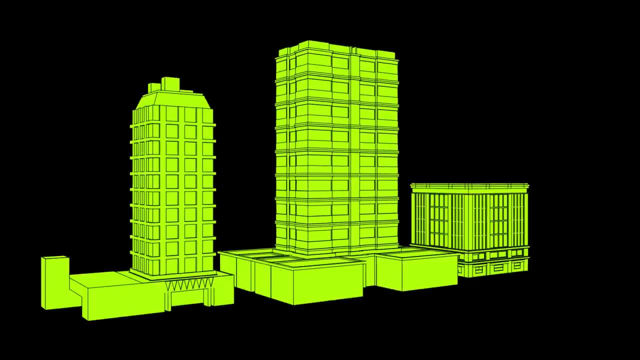 In the case study interview, employers are often looking for strategic thinking, analytical ability, common sense and creativity. In return, you'll get a deeper insight into the type of work an organization does Generally. you'll be presented with an example business. 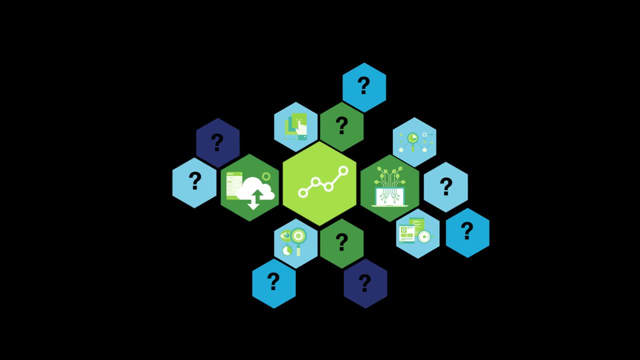 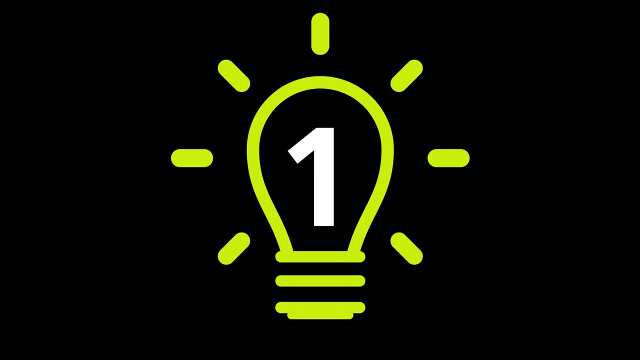 situation and asked a series of questions. The interviewer wants to see how you connect the dots and arrive at a suggested plan of action. These five tips can help One. if there's anything you don't understand, ask clarifying questions, but make your questions. 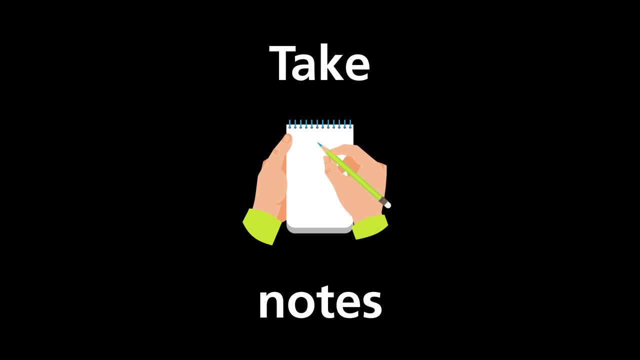 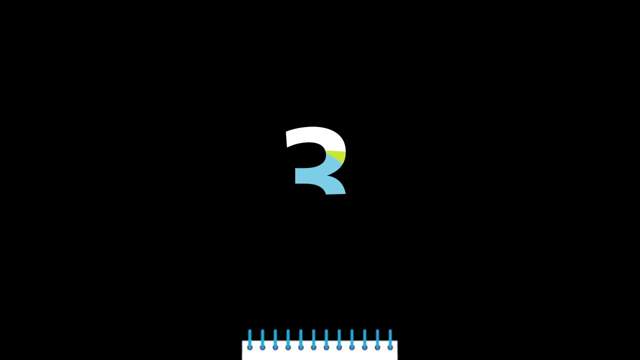 as specific as possible. Two: take notes throughout to make sure you have all the information. It shows you're paying attention and can help guide your thinking. Three: take the time you need. You aren't expected to have all the answers ready. It's better. 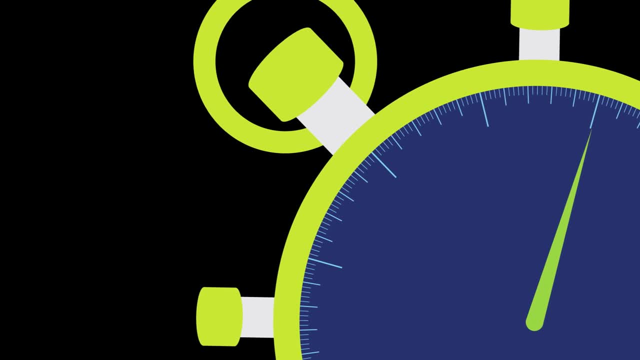 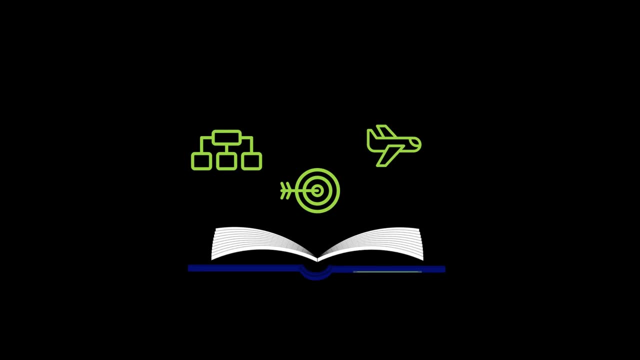 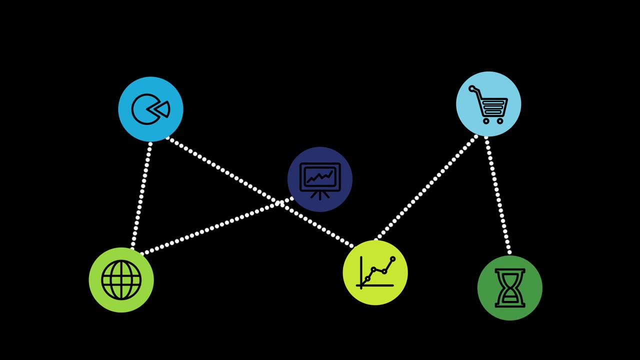 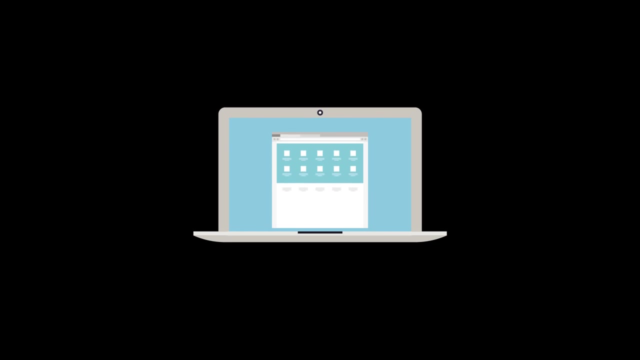 to stop and think rather than just start talking. Four: frame your initial hypothesis as a clear, logical story. This shows your ability to present information. Five: walk the interviewer through your thinking to show how you make sense of complex information. You'll also find example case studies on our careers website.